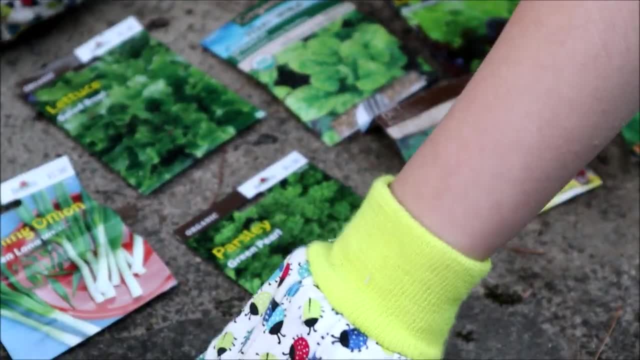 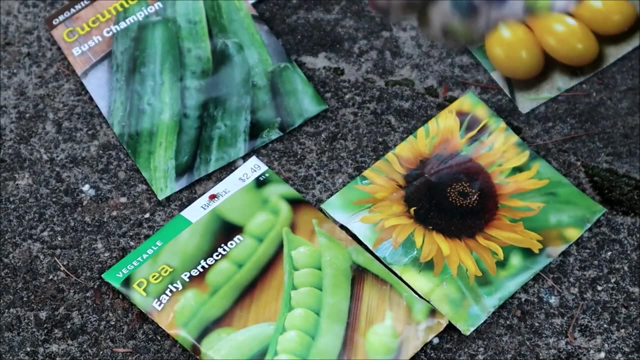 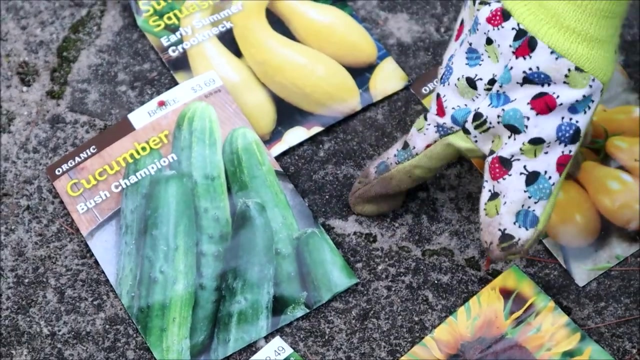 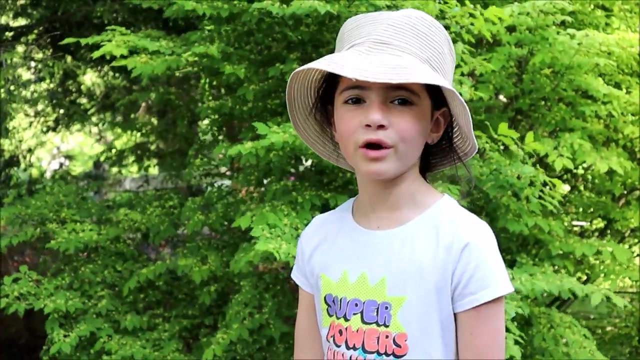 dill and more parsley, and some yellow tomatoes and sunflower and, last but not least, the sweet- oh, this is the one that's last but not least, the cucumbers. So this is what the garden looks like when I haven't planted anything yet. This is what the garden looks like after two weeks. 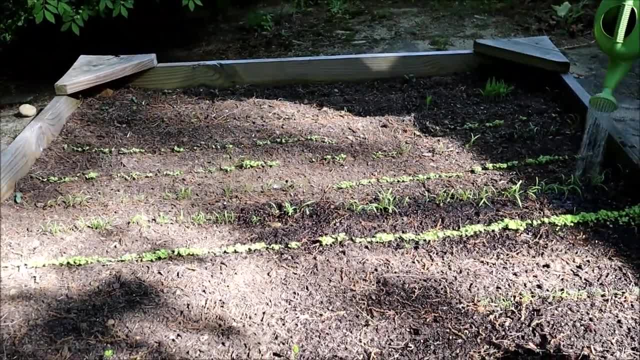 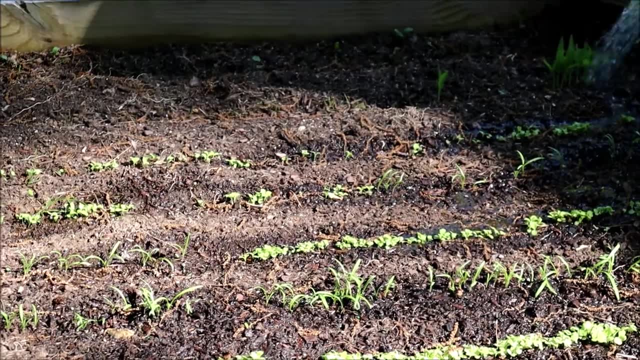 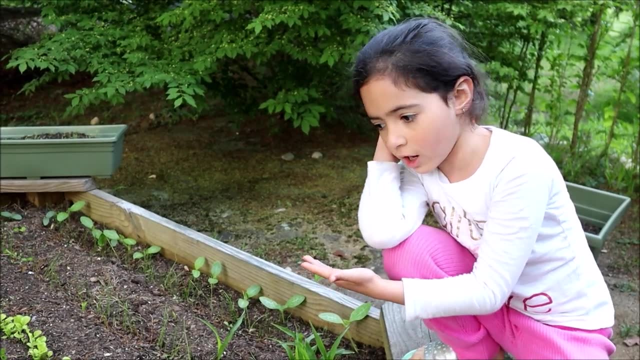 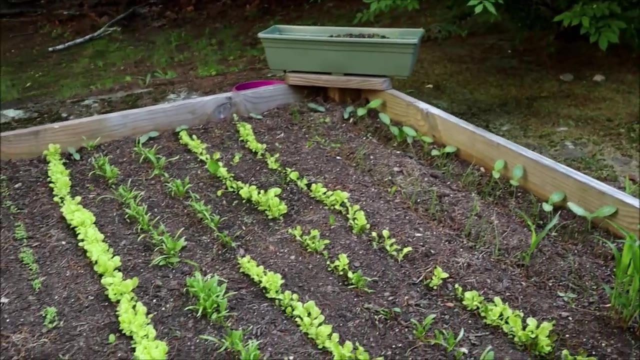 You can see, the seeds can grow up to 7 to 10 feet deep, and if you want to see better results from just flowering your plants, I have a recipe for you too on my website. I think you can start planting right now. 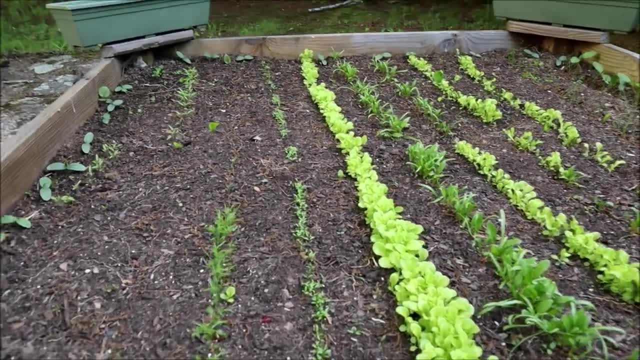 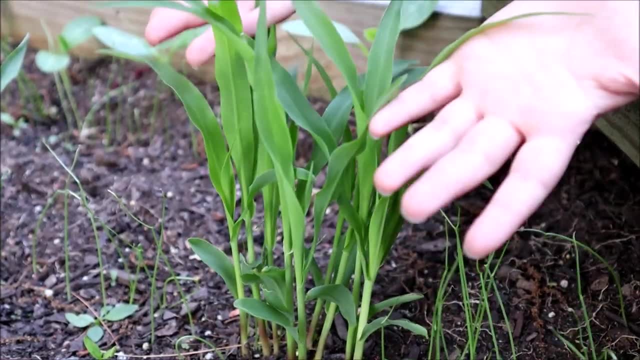 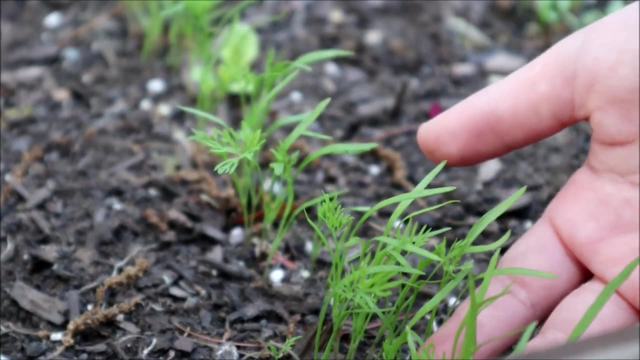 Three weeks later. Whoa, we've been waiting a very, very long time. How much long do we have to wait? Let's see, This is squash, corn salad, spinach, this is dill and, last but not least, the cucumbers. 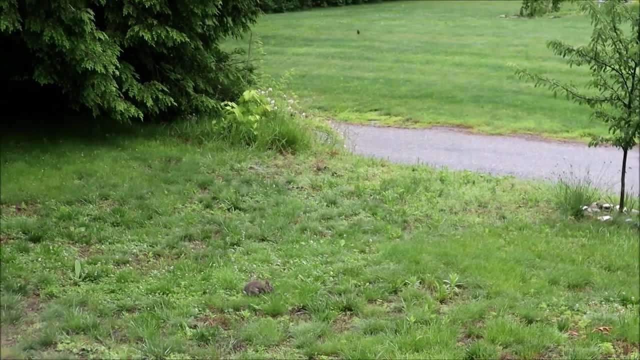 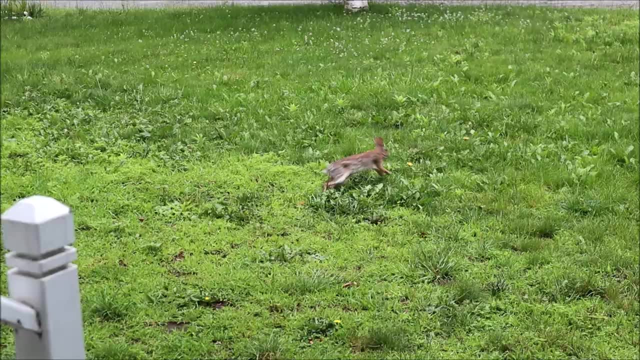 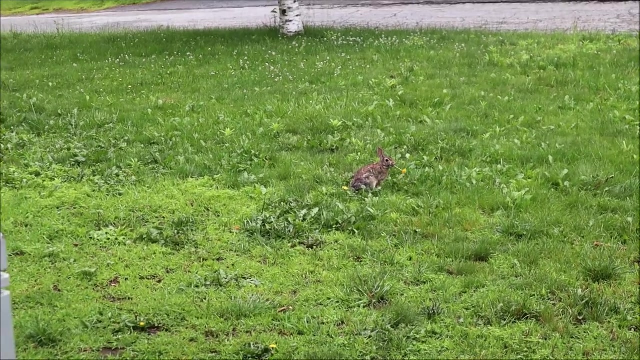 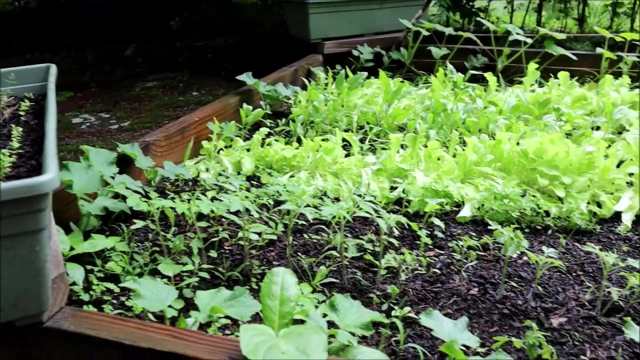 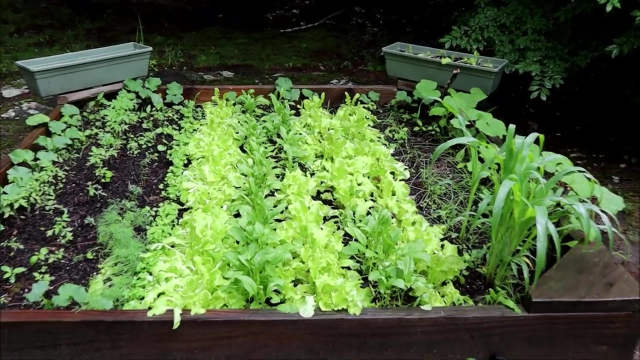 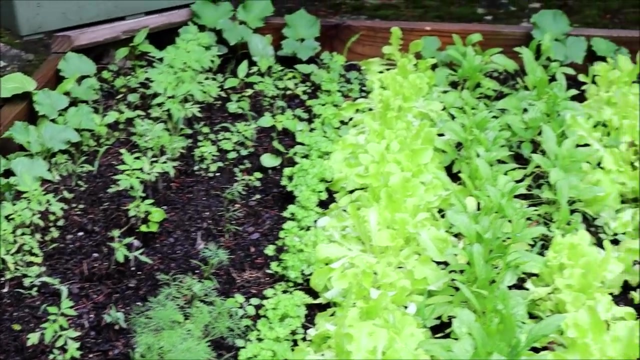 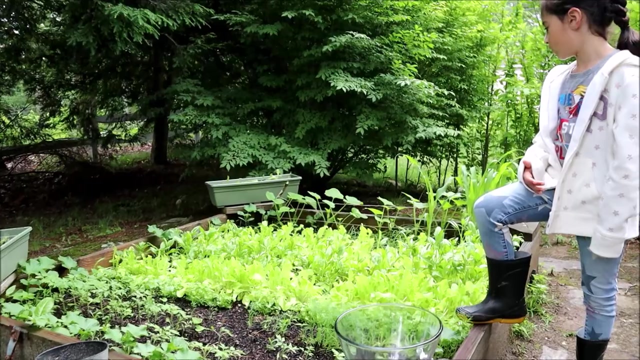 Oh no, there's a bunny in my yard. I think he might go in the backyard and eat our vegetables. Oh no, but he's cute. So it's been over a month since we planted this garden. Everything's looking absolutely wonderful. 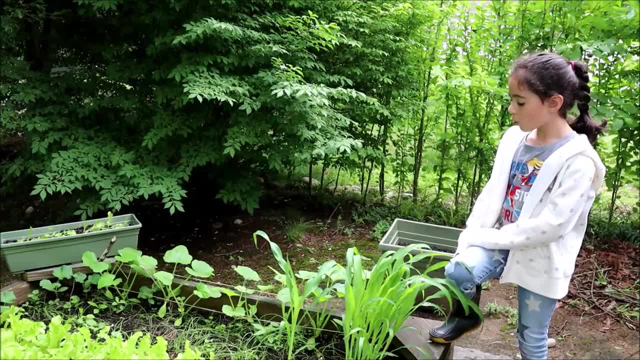 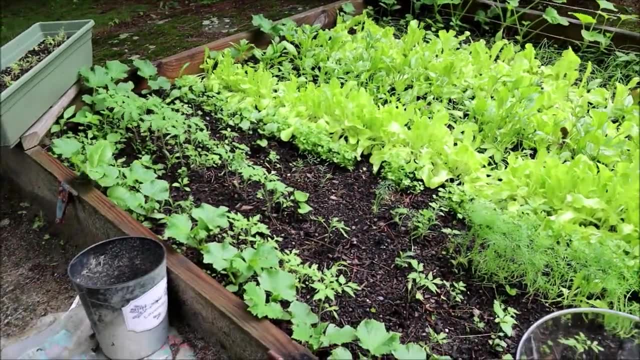 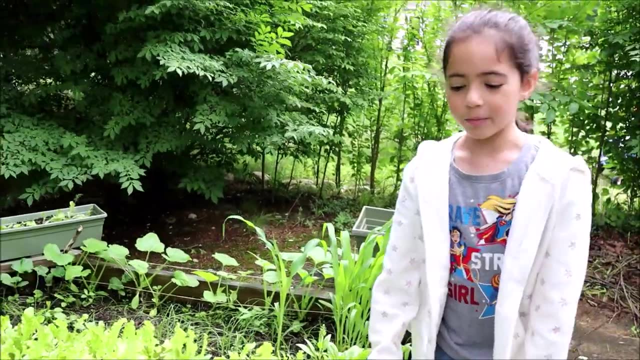 The spinach and salad is ready, So we still have to wait before we pick the corn, the cucumber, the squash and the tomatoes, But my salad and spinach are ready to harvest right now. I'm going to make myself a salad. 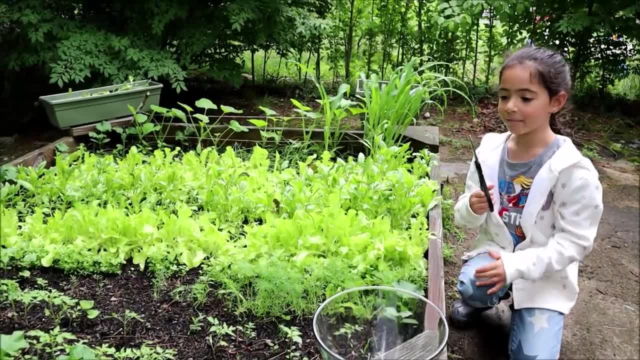 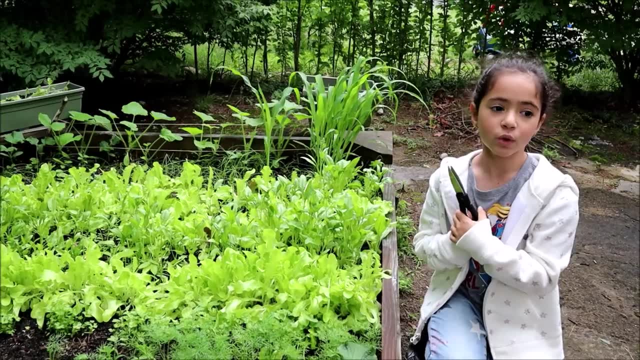 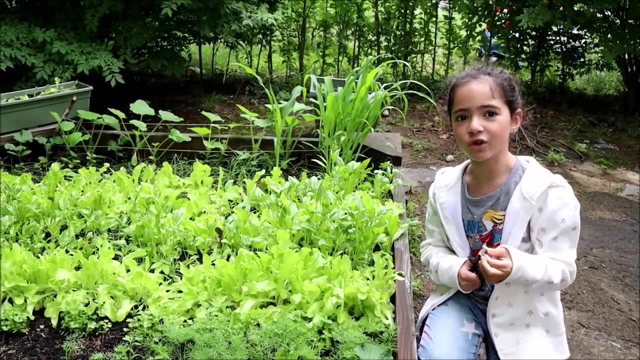 So I have my scissors here and my bowl. But before you use these scissors, make sure you are supervised by an adult so you don't get hurt. So it's fine, because my mom said it's okay and she's right here filming me. 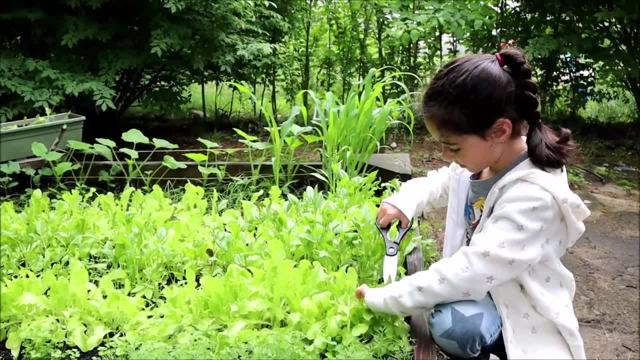 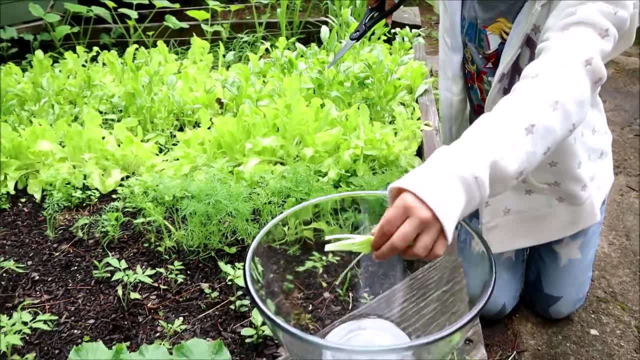 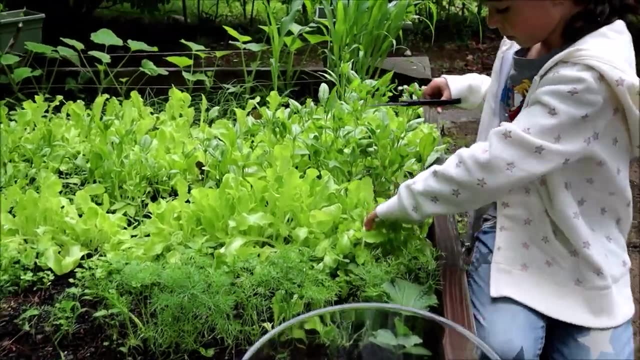 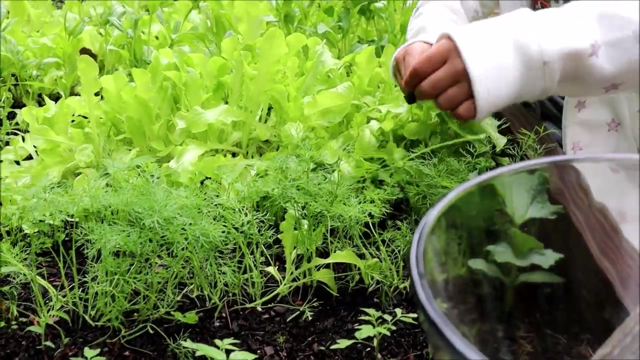 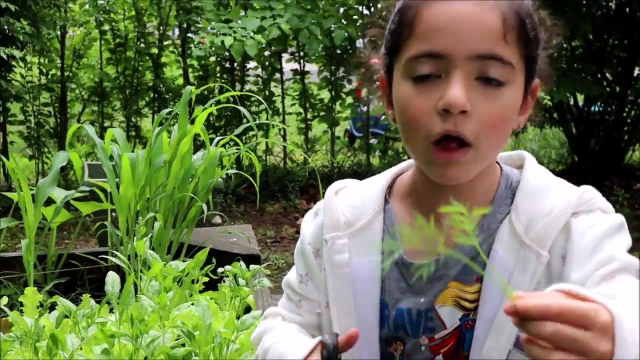 Hey Mom, It's time to cut, So my salad looks like a really pretty salad. My salad looks like chai pancakes or some sort of. I also like some dill on my salad too. I usually like the top of the dill. 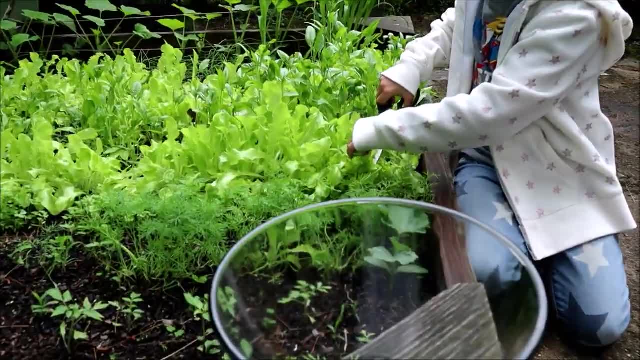 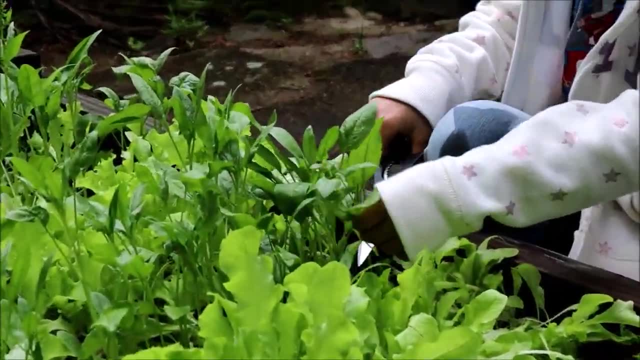 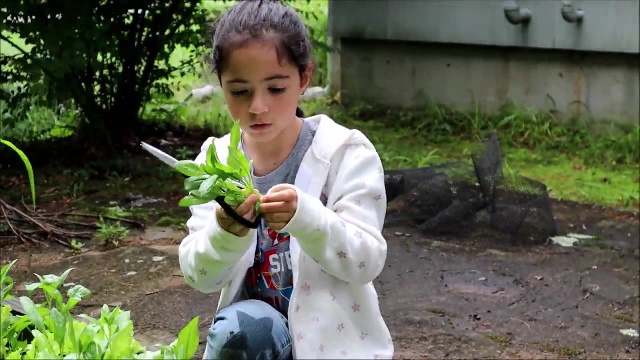 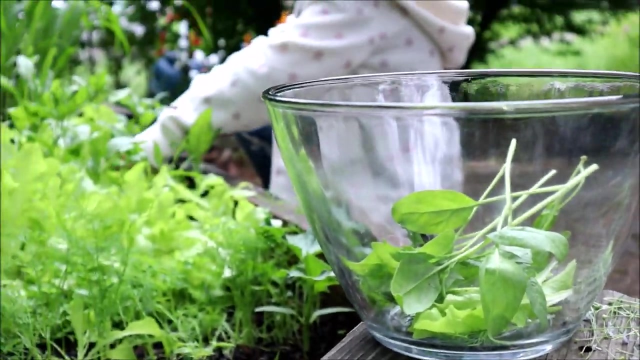 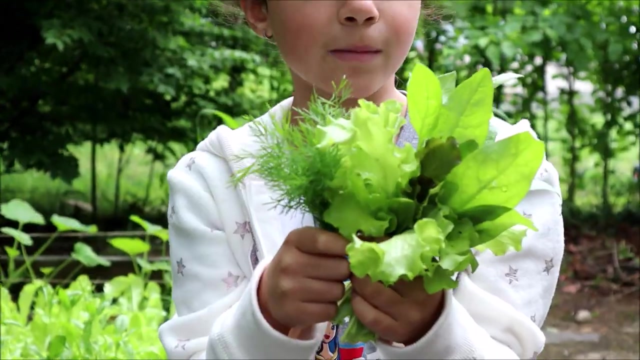 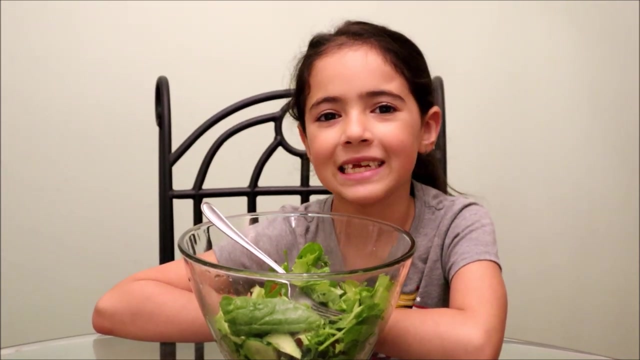 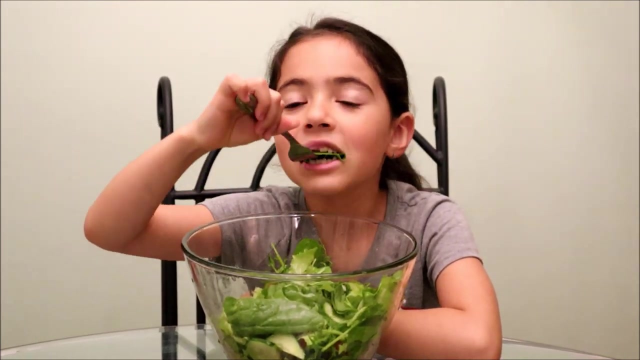 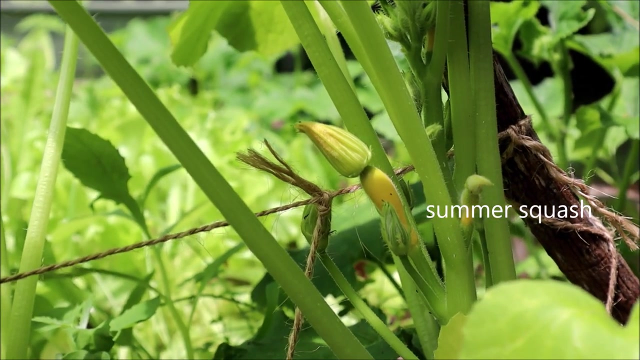 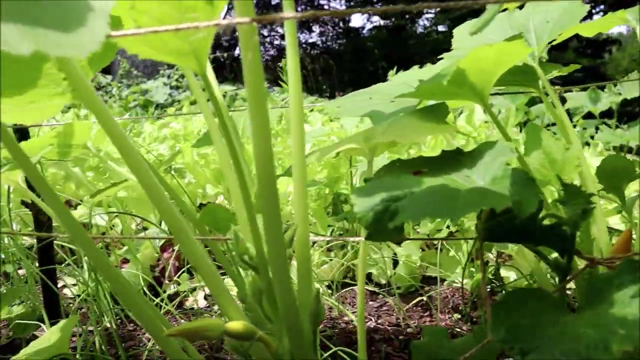 Well, I'll just leave the bottom on for now. We have to wash it anyways, look at these beauties. time to put them in the salad bowl. fresh salad from the garden, ready to eat. Bon Appetit. it's great, this is our garden after three months. 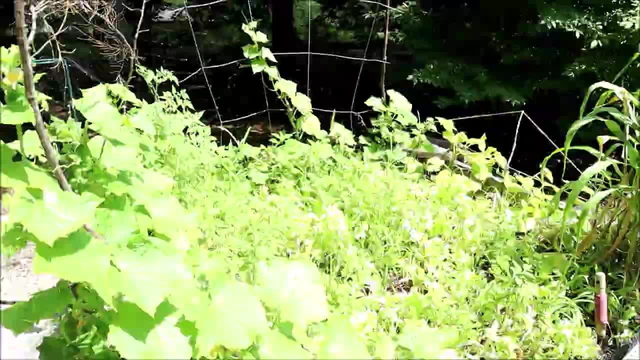 this is our garden after three months. this is our garden after three months. look at our corn. I think we're going to look at our corn. I think we're going to look at our corn. I think we're going to be able to harvest it in the beginning. 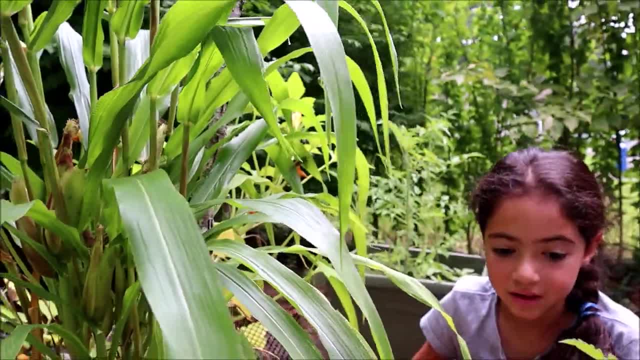 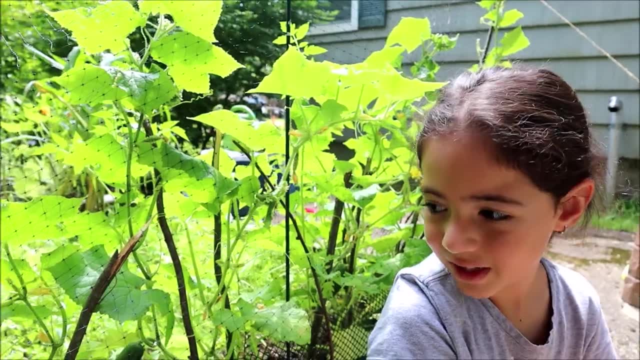 be able to harvest it in the beginning. be able to harvest it in the beginning of fall. look at our cucumbers right now of fall. look at our cucumbers right now of fall. look at our cucumbers right now. they're ready to harvest. 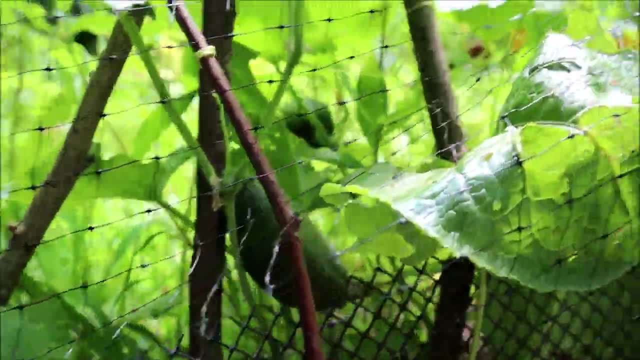 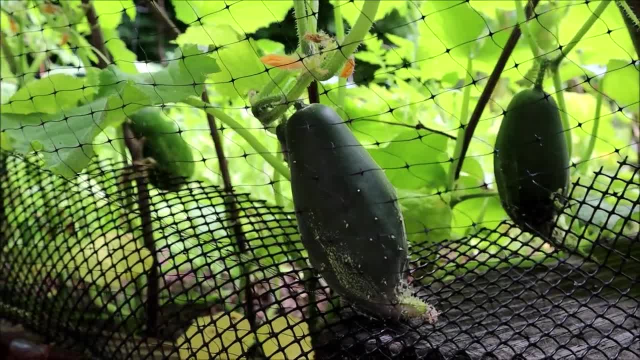 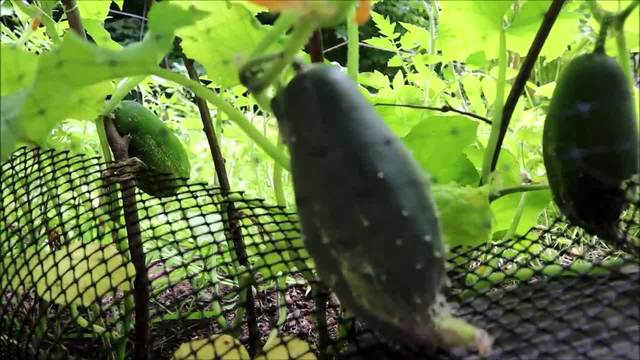 they're ready to harvest. they have a really funny shape. they're ready to harvest. they have a really funny shape. that's because they're getting old. that's because they're getting old. that's because they're getting old. we should pick them before they get too.